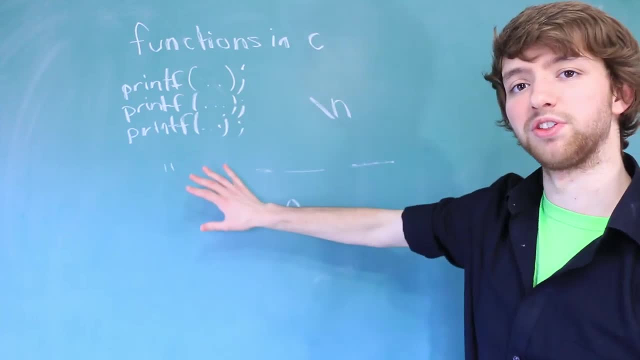 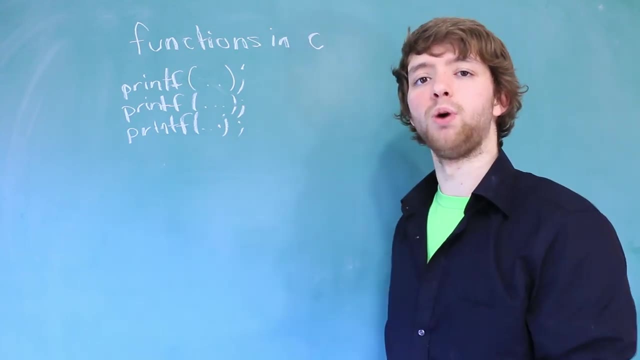 and a bunch of backslash n's. It's harder to consume this with our eyes than smaller printf statements. In addition to this, we've also created code that is going to monitor some kind of information, And we want to continually print out the same statements with new, updated. 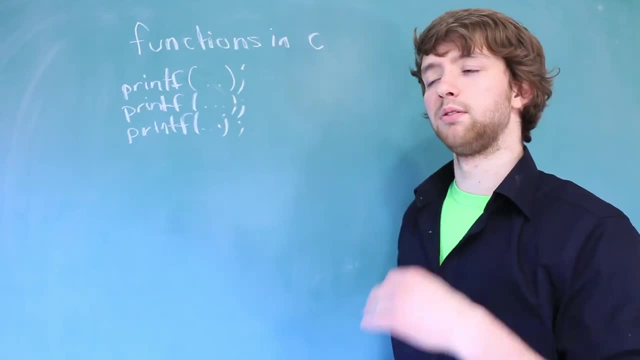 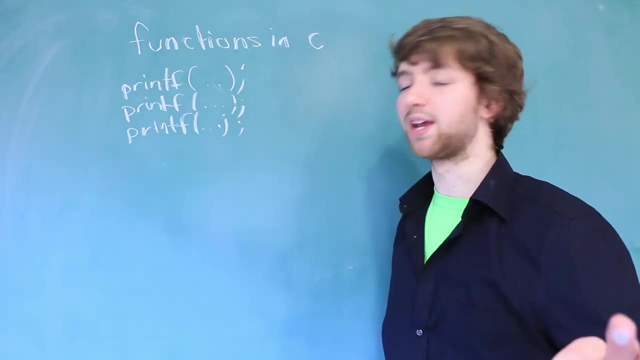 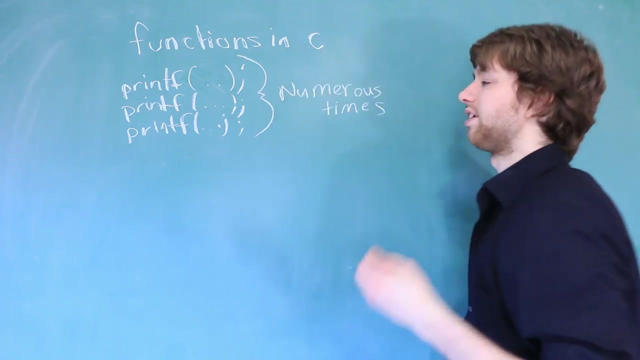 information. So we might have some kind of sensor that this will print like temperatures or something like that. It doesn't really matter what we're using this for, Just make up something in your head. Essentially, we want to execute all three of these numerous times. Well, with a. 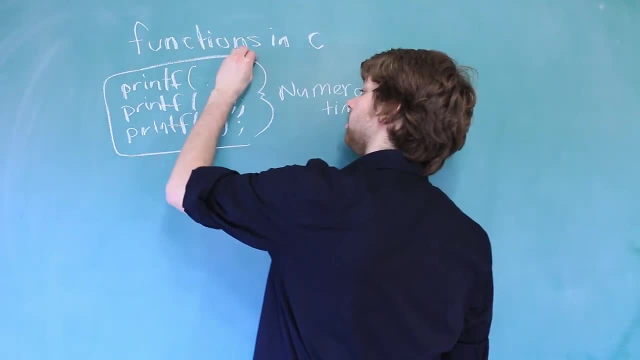 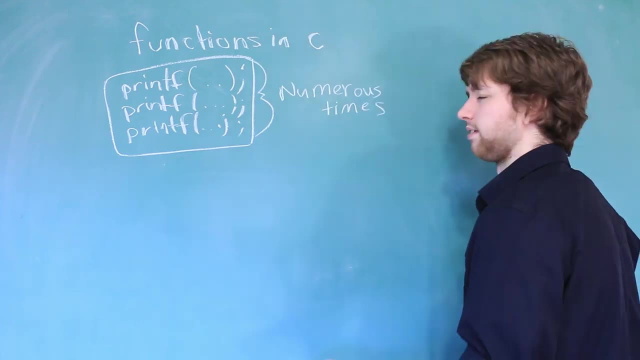 function. we could basically group all three of these together into one. Don't look at me, all innocent, You just ruined my video boy. I don't even know what I was saying. Anyways, you could execute all three of these at one time and give it some kind of name, like. 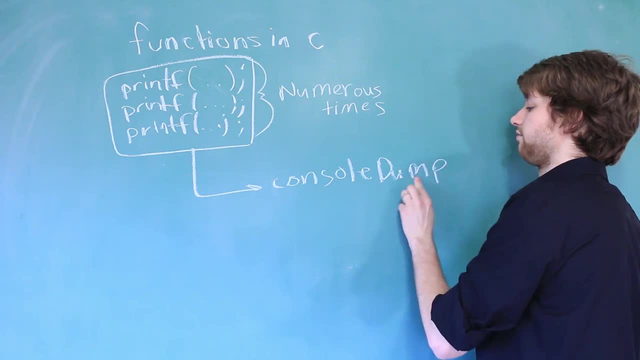 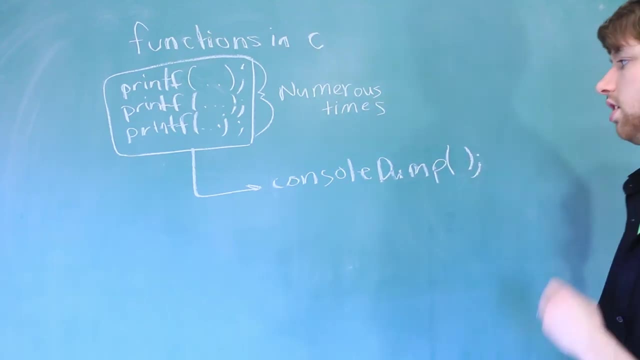 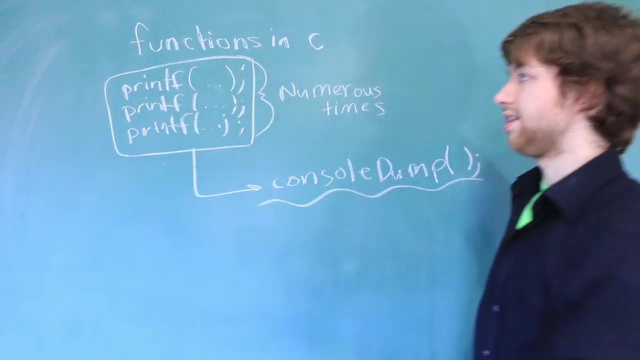 console dump. We're just dumping all the information straight to the console And then we can just call that using these parentheses. That is essentially what a function is. It's a shorthand to calling a bunch of statements. So this here, this printf statement, this is actually a function itself. You can see, we're 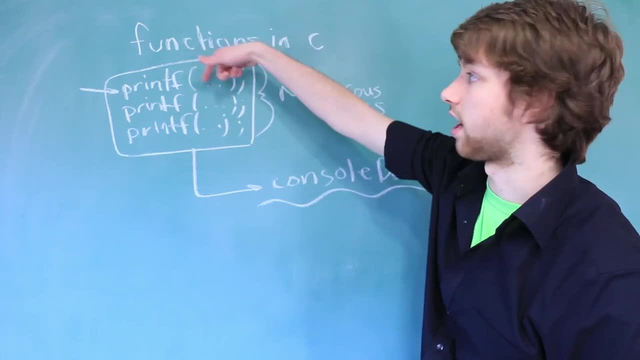 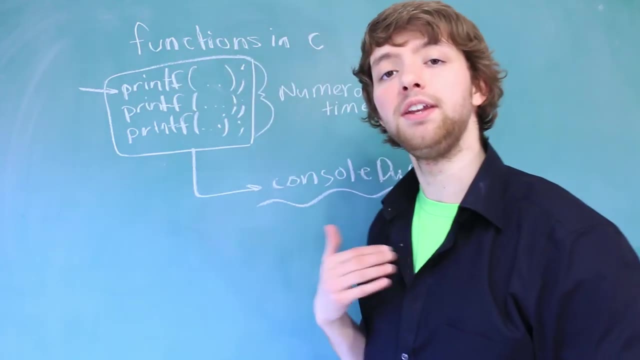 calling it with these parentheses and we're passing in information inside of these parentheses of what we want to print, The actual code for the printf statement. we don't need to care about that. All we need to know is how to use that function. Who knows how many lines of code that function? 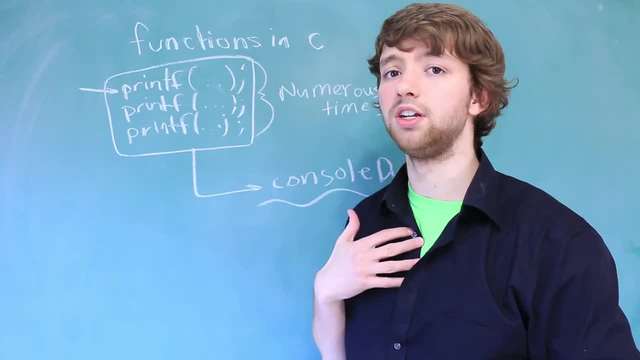 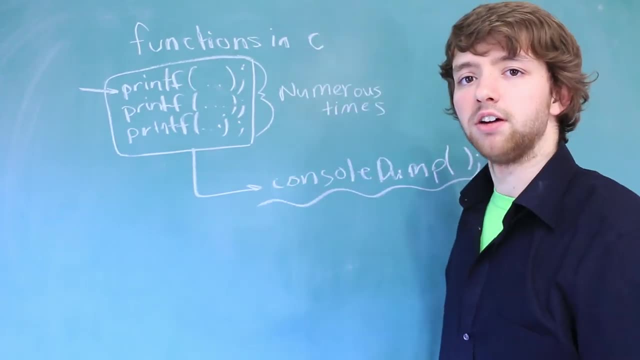 actually takes up. It doesn't really matter to us. to be honest, All we need to know is that when we call this function and pass in some information, it goes to the console. That's all we care about. The second benefit of functions is that if you wanted to change something, 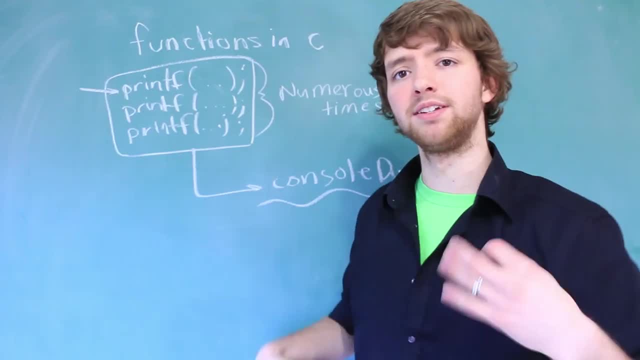 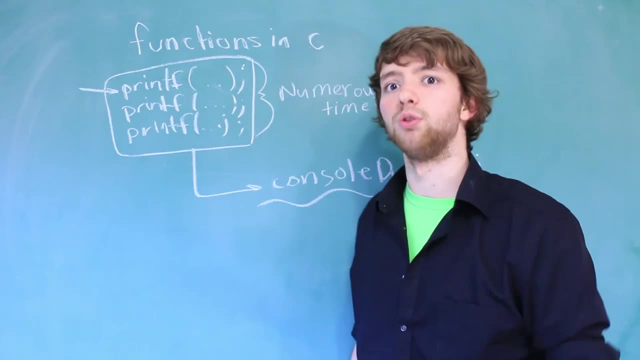 like, let's say we have this code in our program 10 times and we're not using a function and then we want to go back and change something. we're going to have to change it in 10 different locations. That's not going to work very well. 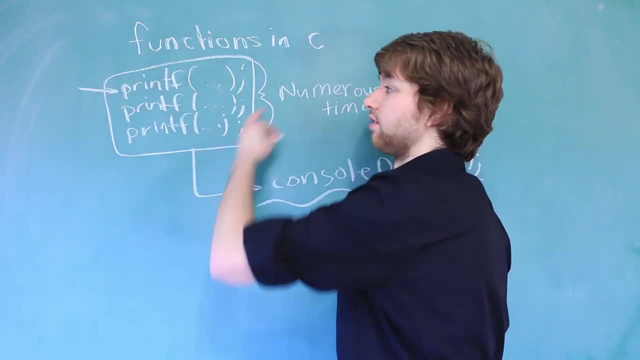 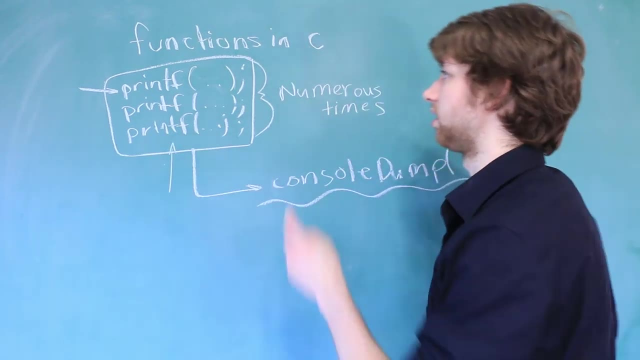 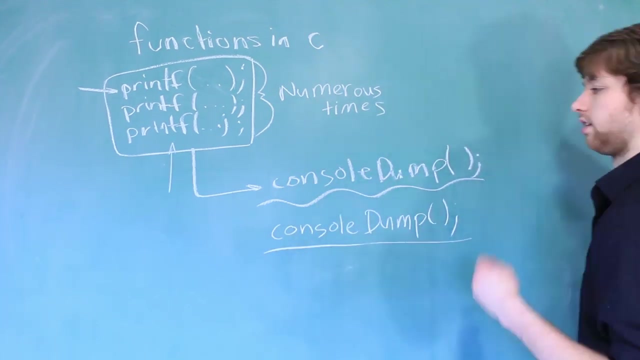 If we're using functions, we can kind of think about it as extracting this code as a formula, and then we only have one copy. So this is our individual copy, and then we can call it multiple times. So now we have two calls and we could repeat this as many times as we wanted. 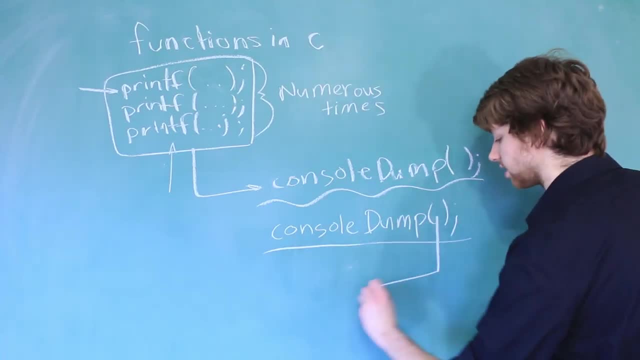 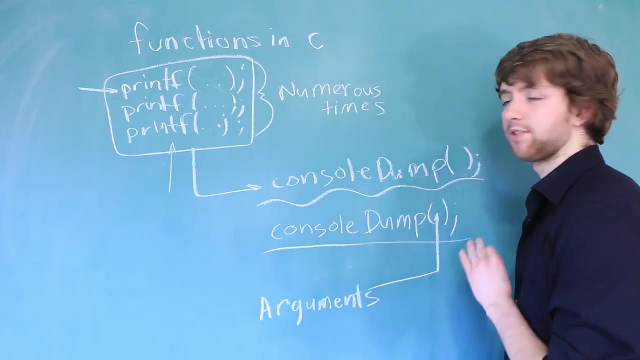 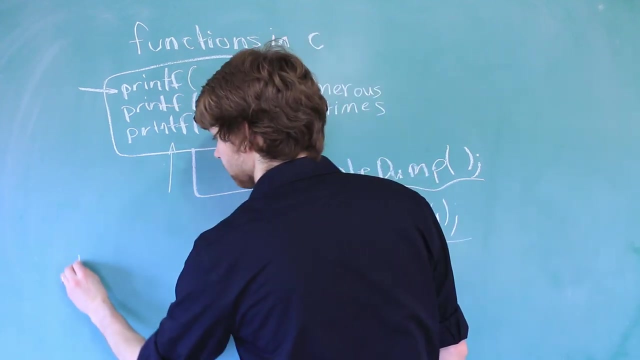 The data that we actually pass into a function inside of these parentheses. these are known as arguments. Functions can accept as many arguments as they want. The only thing is you have to separate multiple arguments by commas. So, for example, in this printf function we could do something like this: where x is the name of a. 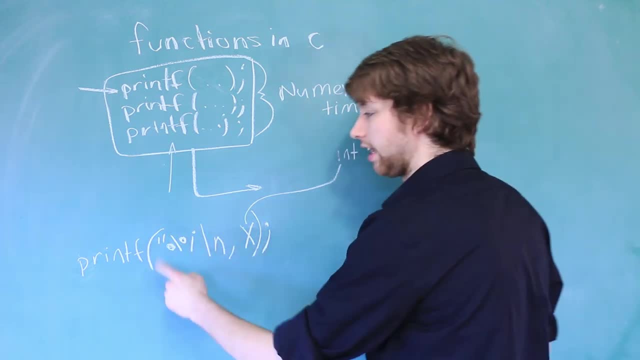 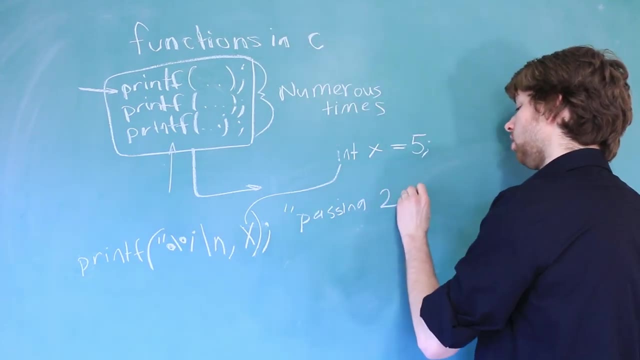 variable that stores some value. The action of putting data here is called passing. So if you had to put it into a sentence you would say: we are passing two arguments, The arguments in this case. the first one would be this string here: 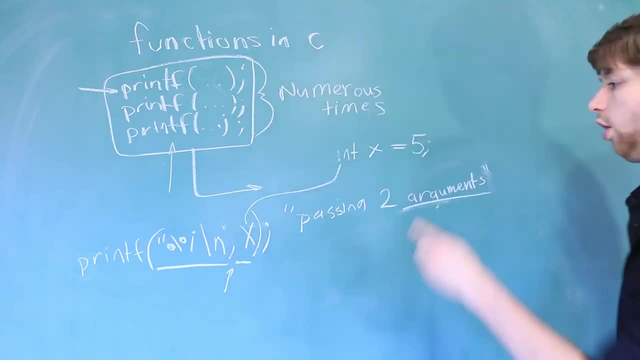 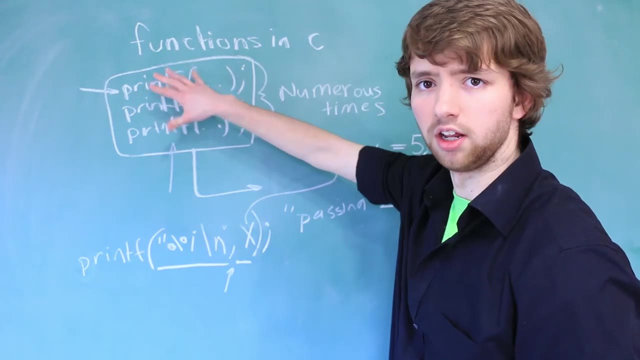 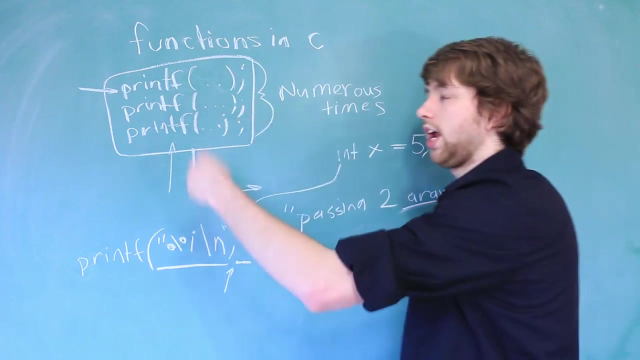 the second one would be x and they're separated by a comma. Arguments allow us to customize our functions. For example, in this situation where we had this function we created, called console dump or whatever, we could accept arguments that allow us to change how the function works. 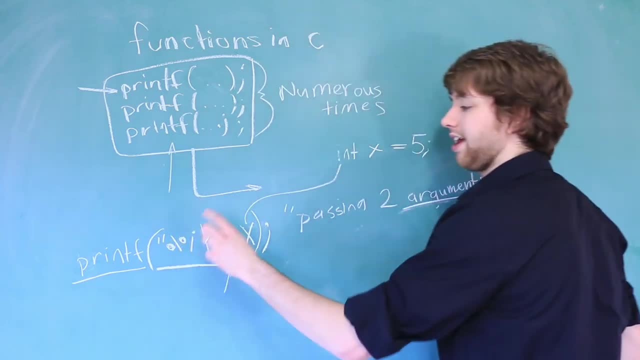 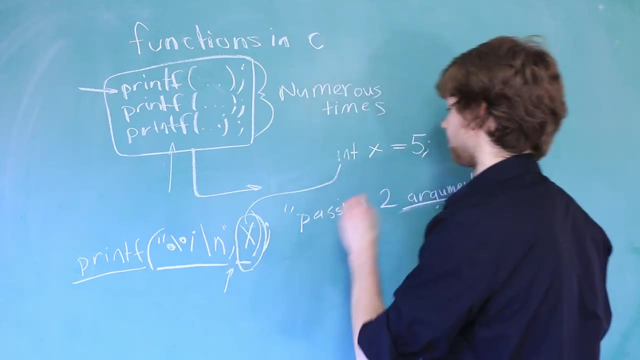 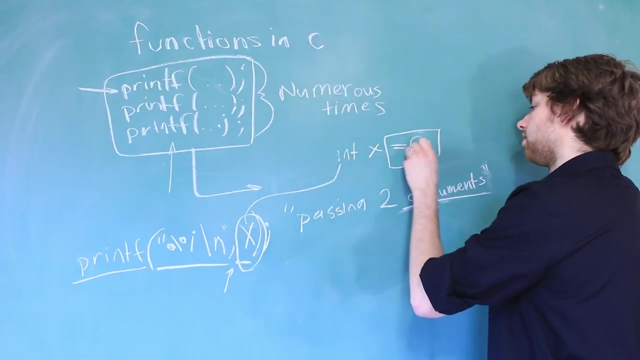 You can see that in the printf function. The printf function does something different depending upon what we pass in. If we're passing in x here and it has the value of 5, it's going to print 5 to the console. But if x has the value of 6, it's going to print 6.. 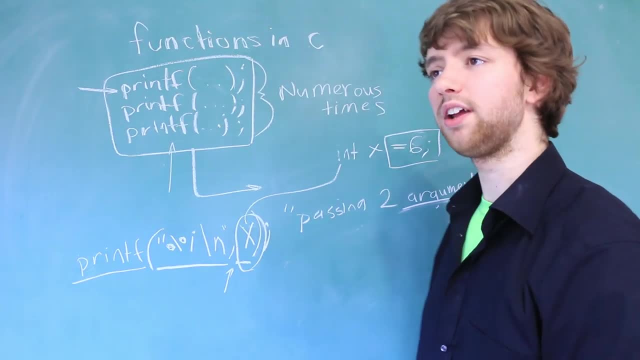 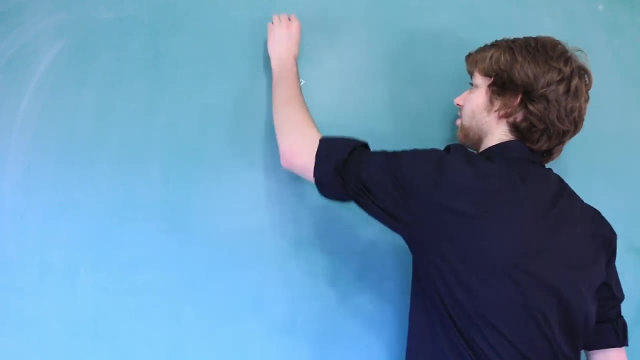 So if you need another way to think about this, you can think of functions kind of as cookie cutters, right? So let's say we have this cookie cutter in the shape of a carrot. This could be our function. A cookie cutter only gives you most of what you need. As for the actual 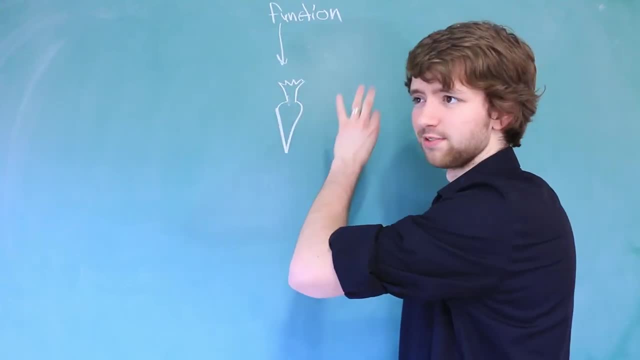 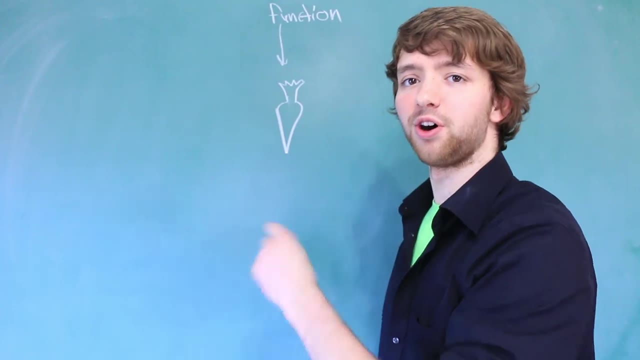 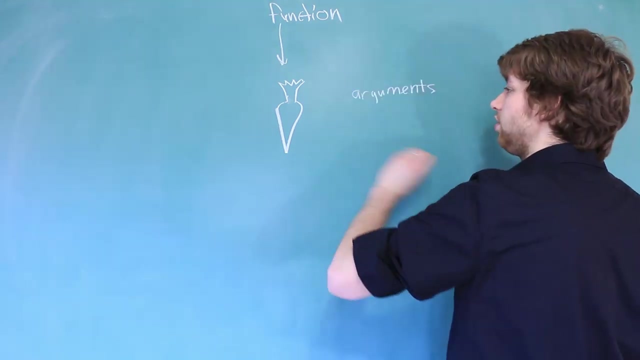 color and the material material. you're probably going to use this for eating, so I don't know if material would be the best word. but substance, all of that stuff depends on you. You get to choose that kind of stuff. You can think of that kind of stuff as the arguments You could easily 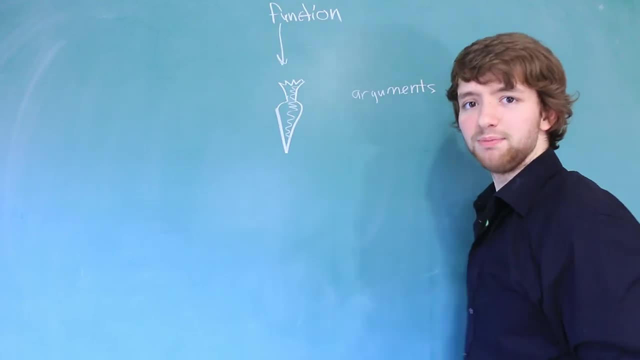 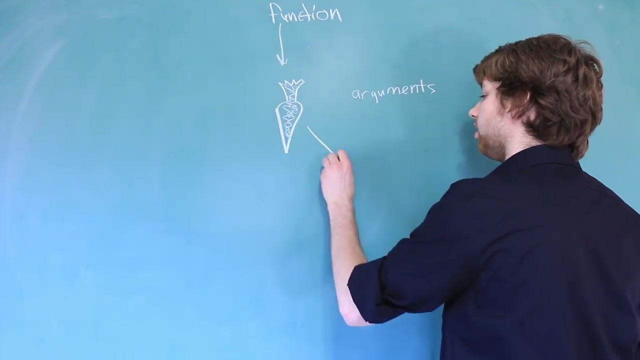 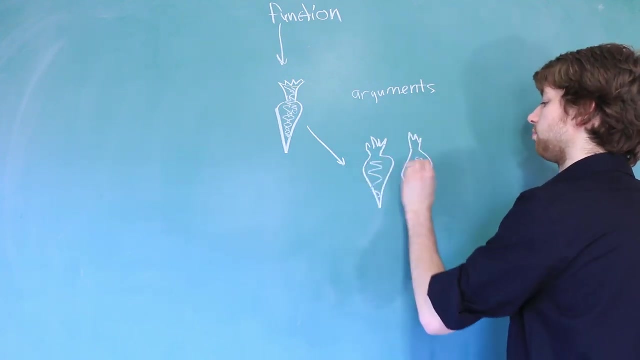 fill this up with peanut butter and then make a carrot-shaped peanut butter cookie, or you could fill it up with chocolate chip cookies. The end result: it looks like a carrot, but each carrot is slightly different. This one could be, you know, chocolate and this one could. 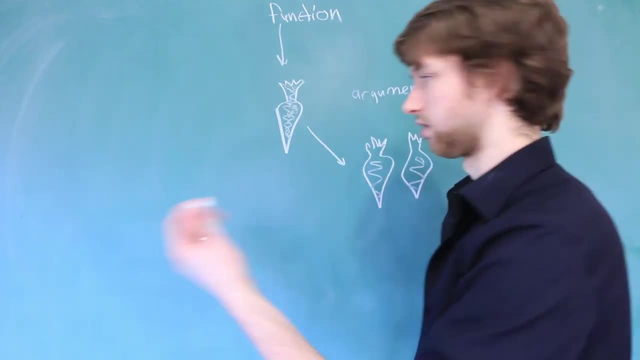 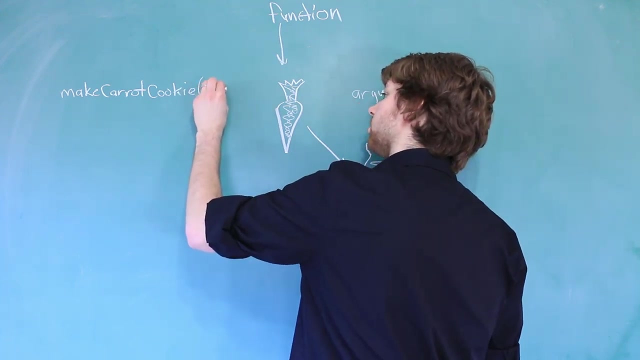 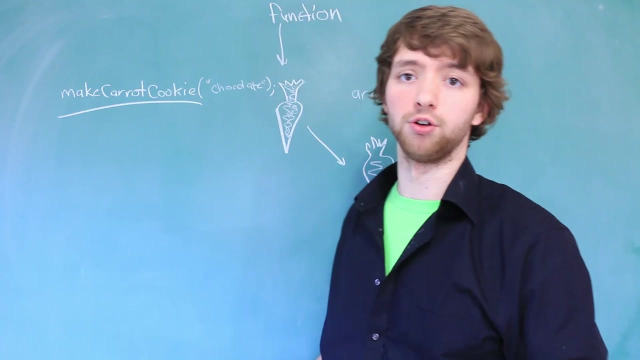 be peanut butter. If you had to convert this into computer science terms, it would look something like this: Make carrot cookie, and then we could pass in here like a string, for example chocolate, Where this function is defined. that's what we'll get into farther in the series when we talk about creating our own.